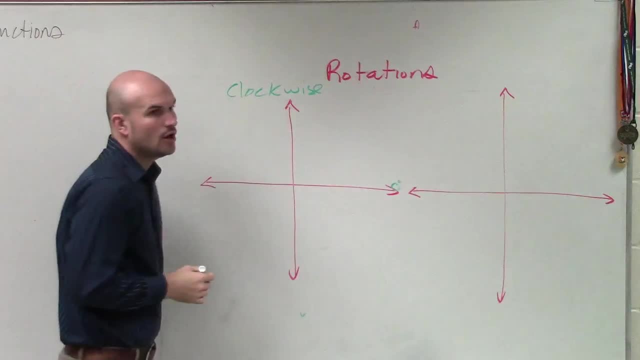 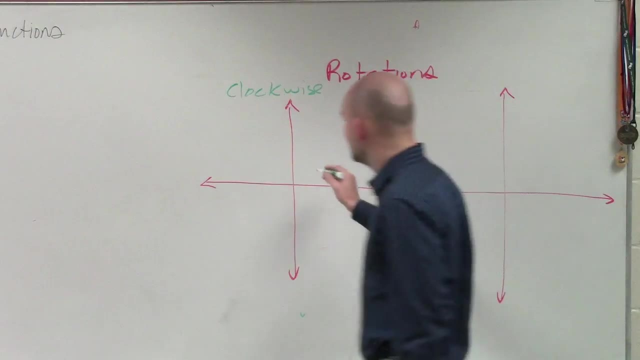 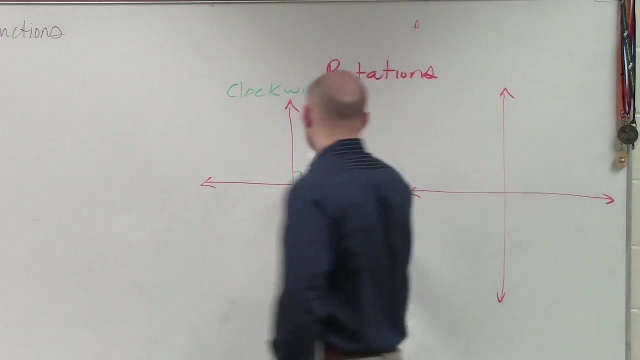 do clockwise. Now hopefully you guys know when we have our coordinate system. our coordinate systems are perpendicular to each other. Therefore they create a 90 degree angle. Our x and our y-axis are perpendicular to each other. So we can say: if I rotate something, if I rotate. 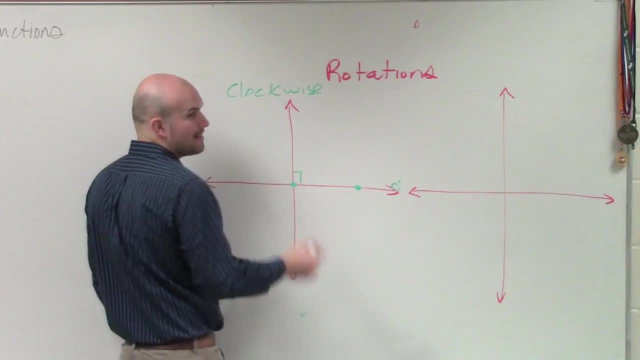 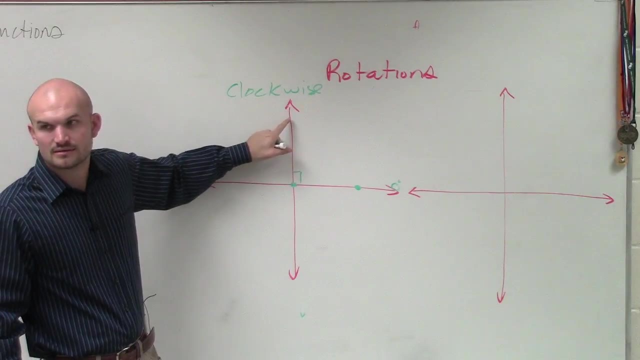 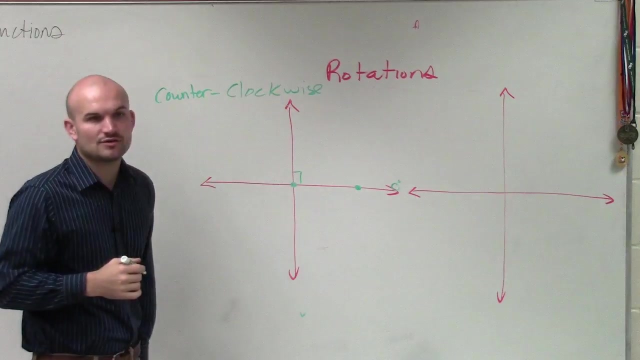 a point. let's say there's a point on this line- and that's going to be my point- that I'm going to rotate on. If I rotate my point from here to here, I have rotated at how many degrees? 90 degrees in the counterclockwise direction. So from here to here would be 90. 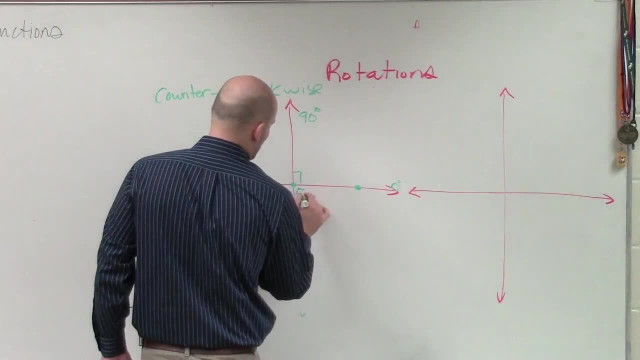 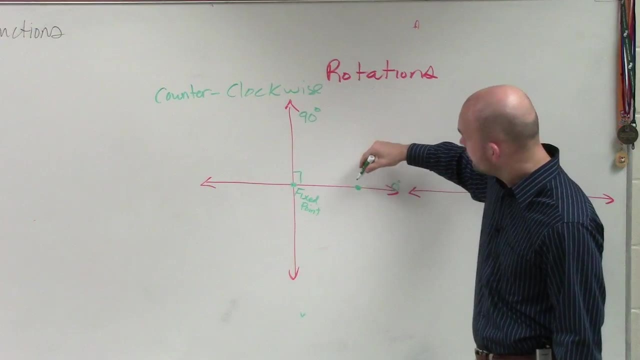 degrees. So if here was my fixed point- this is the point I'm going to rotate on- And if I had a point on this line, if I rotate to it from here to here, I would be over 90 degrees. here to here, that would be 90 degrees. 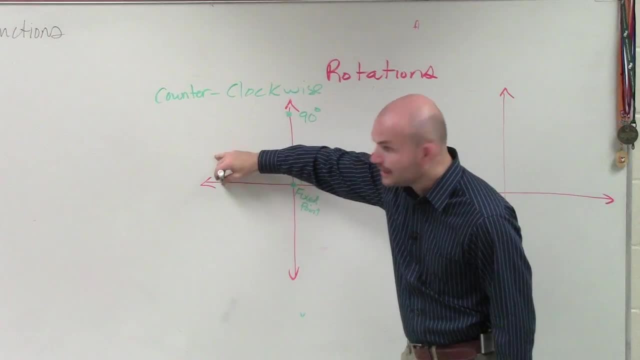 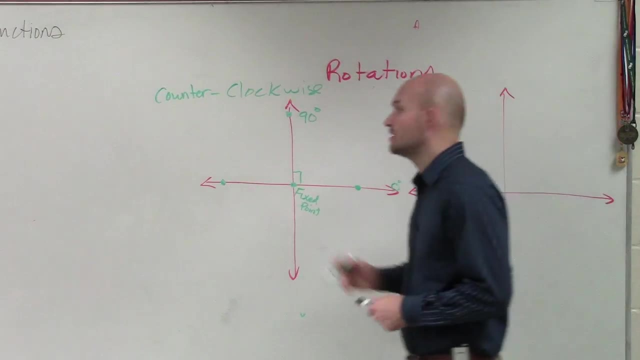 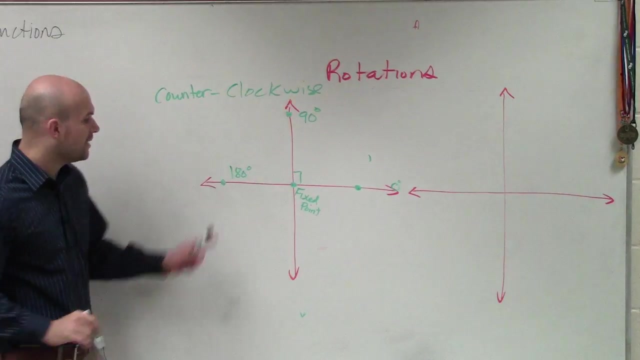 If I rotate the point from here all the way over to here, Mario, how far would that be Exactly? Thank you, Taylor. how far would that be? 180 degrees in the counterclockwise direction. Now again, remember guys, these are all 90 degree angles. 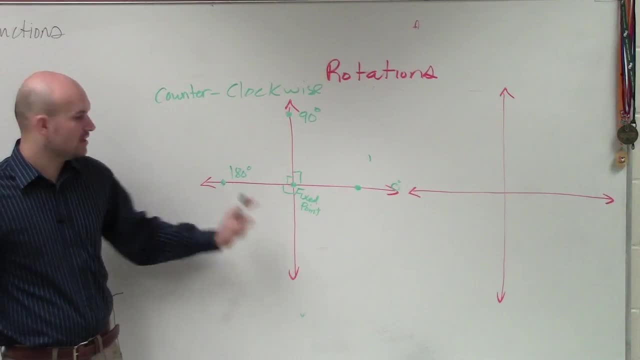 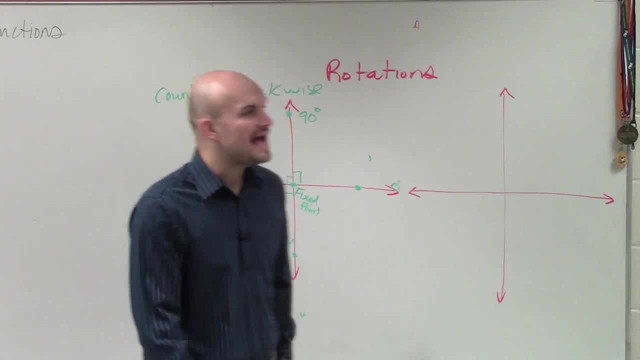 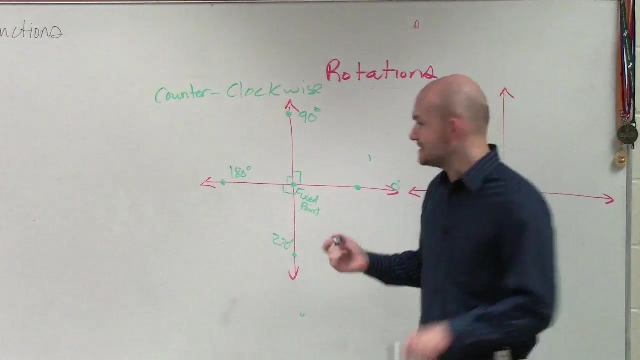 So if I wanted to go from here all the way over to here, well, I just need to add 90 again to 180, which would be 270. And then if I rotate this point about this fixed point all the way around, it's going to give me the exact same image. 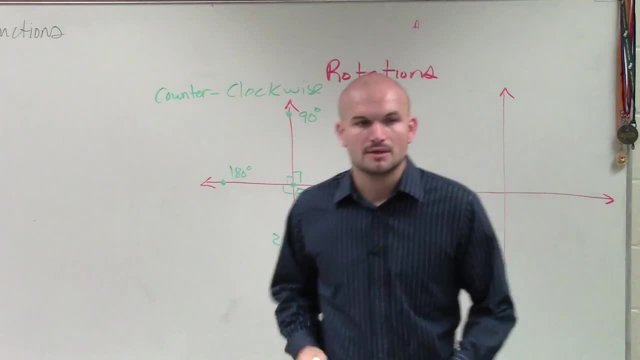 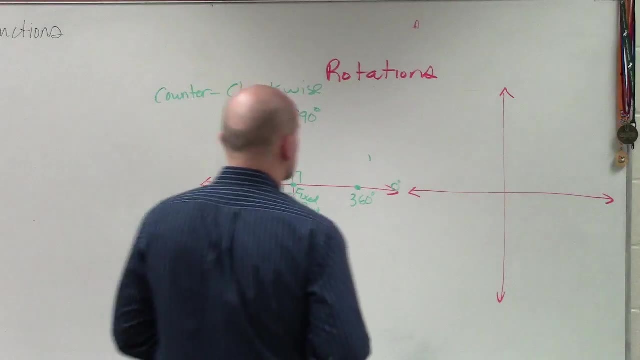 But anyways, you guys will at least know that's 360.. So I'm going to ask you to rotate points counterclockwise And I'm also going to ask you to rotate points clockwise. So what's different, What's different about them is the same thing. 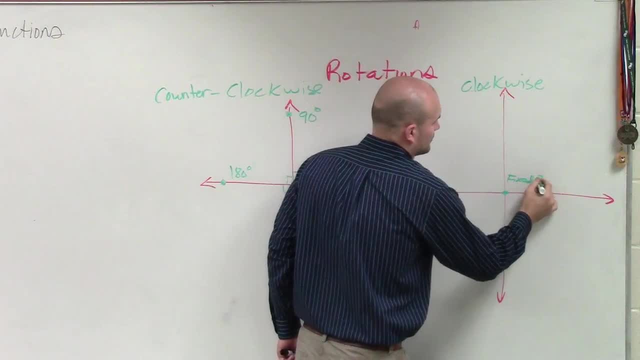 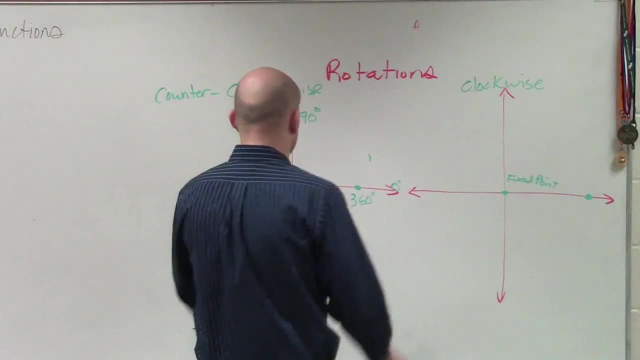 Let's say we have our fixed point And there's the point that I'm going to rotate. If I say, rotate this clockwise 90 degrees, well, up here was 90 degrees but that was counterclockwise, So 90 degrees over here Sam would be where.